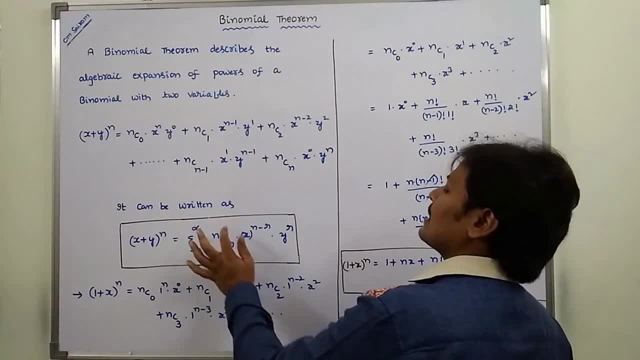 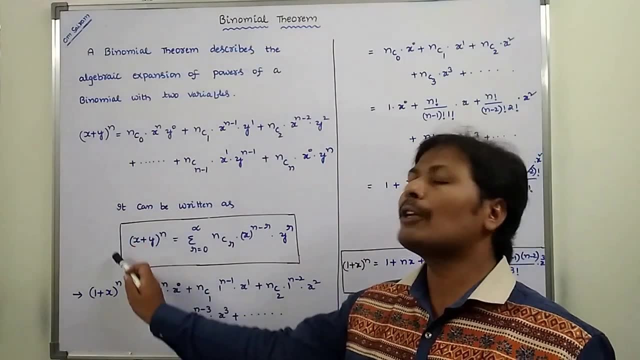 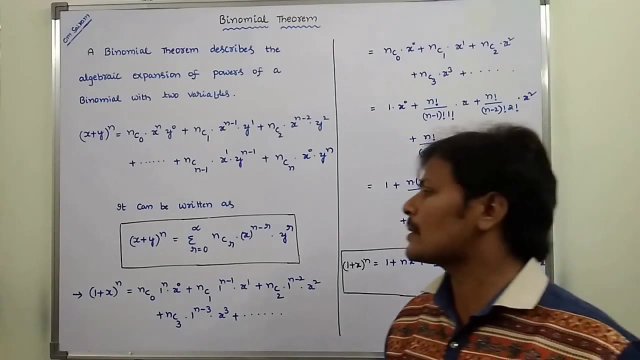 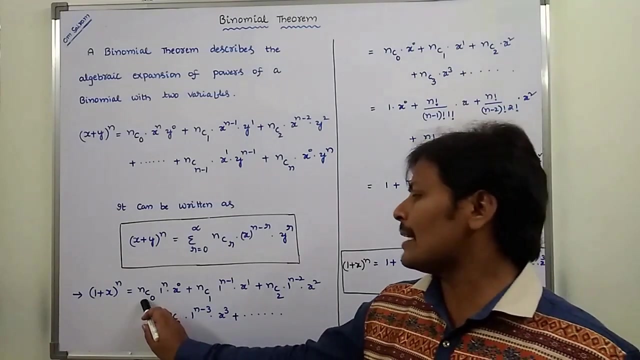 r is equal to 0 to infinity. ncr into x power n, minus r into y power r. Okay, This is the binomial theorem containing two variables. expansion: Okay, Suppose 1 plus x whole power n. So what is the expansion? Okay, So that is: nc0 into 1 power n into x power 0, nc1 into 1 power. 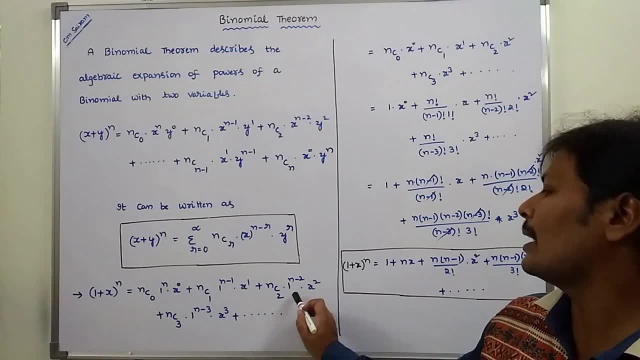 n minus r into y power r. Okay, So that is: nc0 into 1 power n into x power 0,. nc1 into 1 power n minus 1 into x power 1, nc2 into 1 power n minus 2 into x power 2 plus nc3 into 1 power n minus 3. 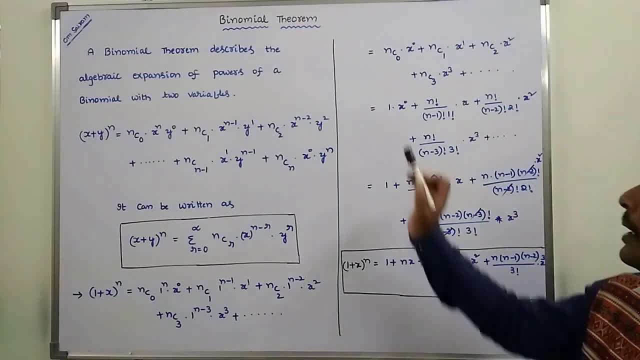 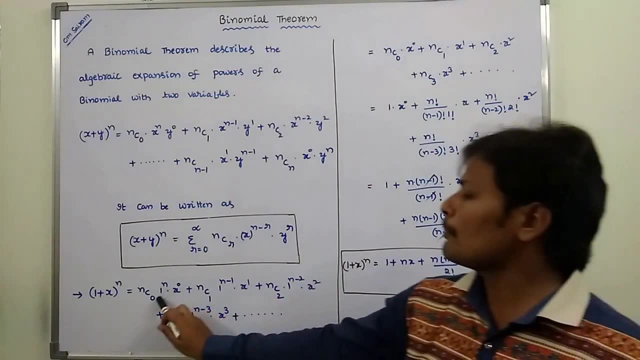 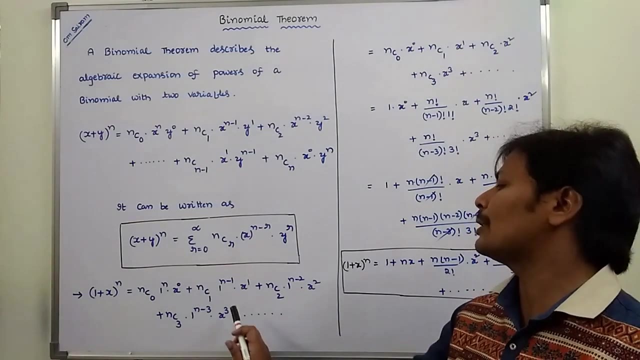 into x power 3, etc. So now 1 power, anything is nothing but 1.. So nc0 into 1 power, 1 is 1.. 1 into x power 0.. That is nothing but x power. 0 plus nc1 into this is 1.. This is x power, 1.. So 1. 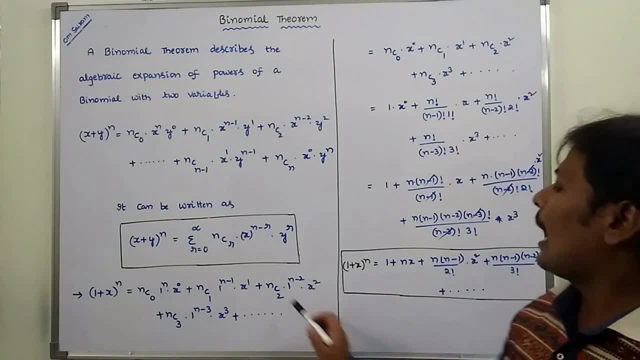 into x power, 1 is nothing but x power. 1. nc2 into 1 power, n minus 2 is nothing but 1.. 1 into x square is x square plus nc3 into 1 power. n minus 3 into x power, 3. So 1 into x power, 3 is x power. 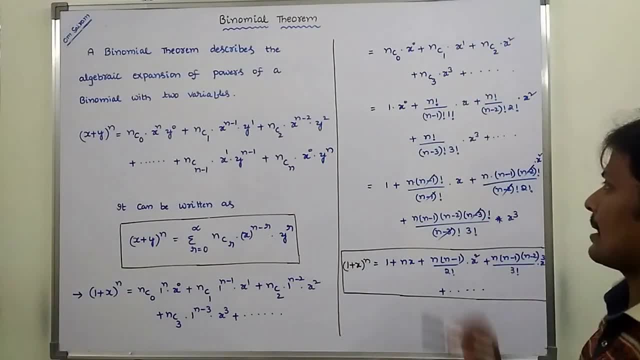 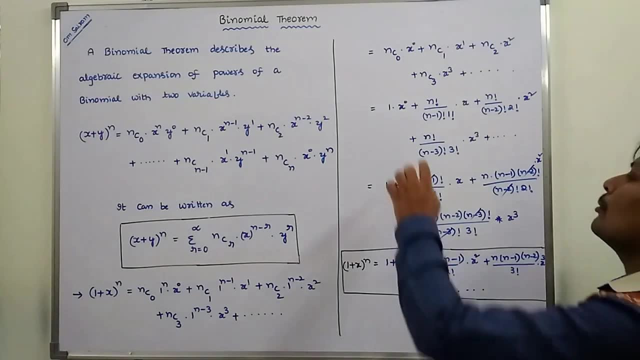 3.. nc3 into x power, 3.. Next So nc0 value is 1.. So x power 0 is 1.. So 1 into 1 is nothing, but 1 into x power, 3.. Next So nc1.. So what is ncr formula? n factorial by r factorial into n minus r. 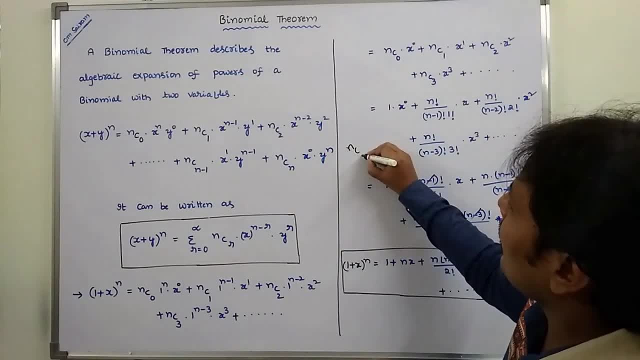 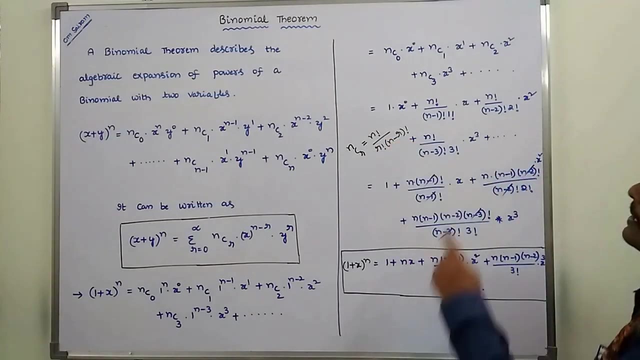 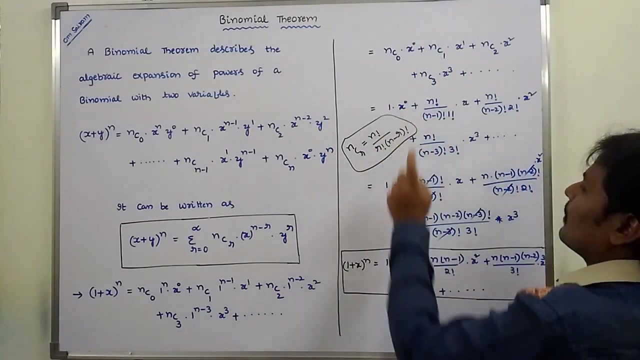 factorial. So here ncr is equal to n factorial, by r factorial into n minus r factorial. Okay, So this is the formula ncr formula. Okay, According to this, so 1 into x power 0 is 1 plus n factorial, can be written as n into n minus 1 factorial, Because 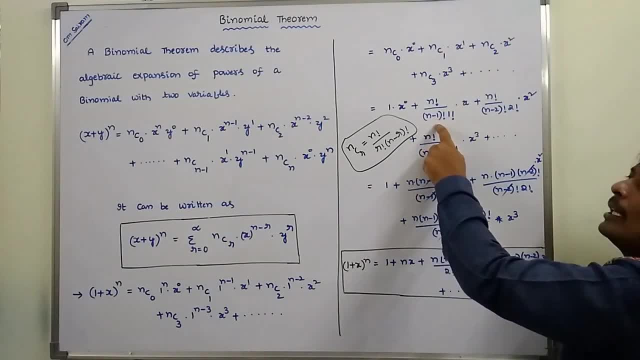 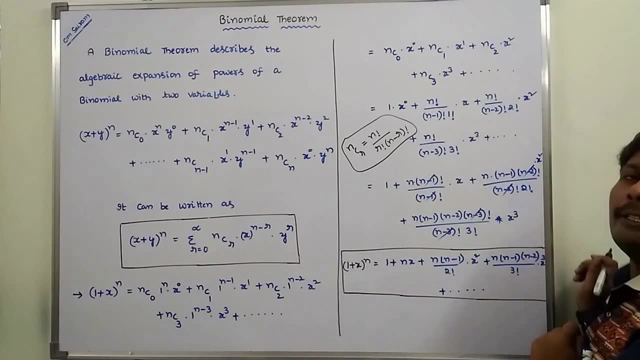 the denominator contains n minus 1 factorial. To cancel this n minus 1 factorial. n factorial can be written as n into n minus 1 factorial. Okay, Divided by n minus 1 factorial into x Here: n minus 1 factorial. n minus 1 factorial. cancel. Then we are waiting. 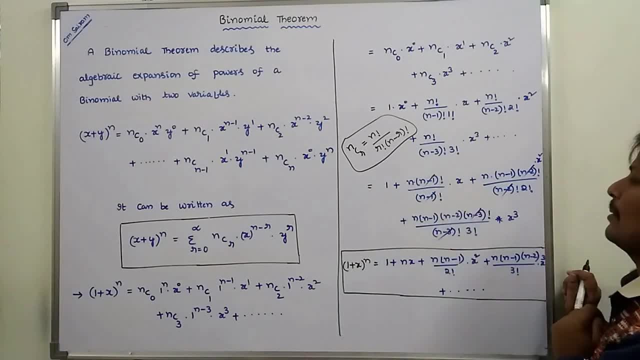 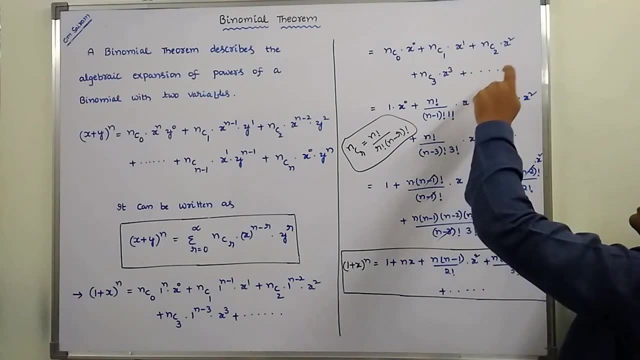 So we see n into xi below 0, n into xi is twice m over 0. So we have the tensile left and tensile opened up And this is what is n into n minus 1 variable is 0. And this one. 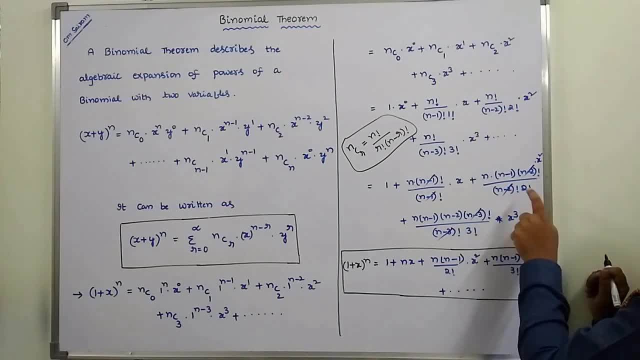 factorial, so divided by n minus 2 factorial into 2 factorial. n minus 2 factorial, n minus 2 factorial, cancel. then the remaining is n into n minus 1 by 2 factorial into x square. next third one: n factorial by n minus 3 factorial into 3 factorial, so to cancel the denominator term n. 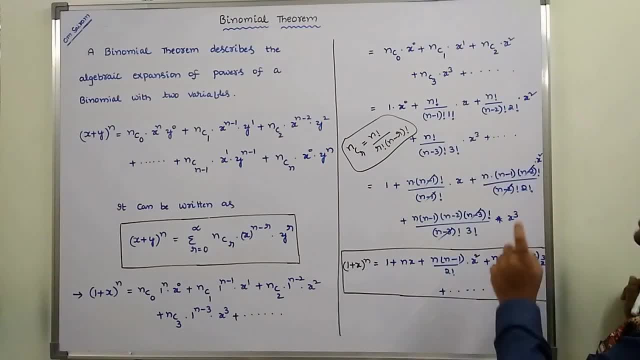 minus 3 factorial. n factorial can be written as: n into n minus 1, into n minus 2, into n minus 3 factorial. so n minus 3 factorial, n minus 3 factorial. cancel the remaining term n into n minus 1, into n minus 2 by 3 factorial into x cube. so finally we are getting this one 1 plus x whole. 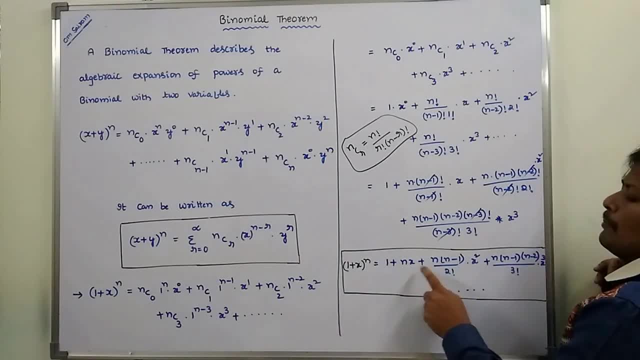 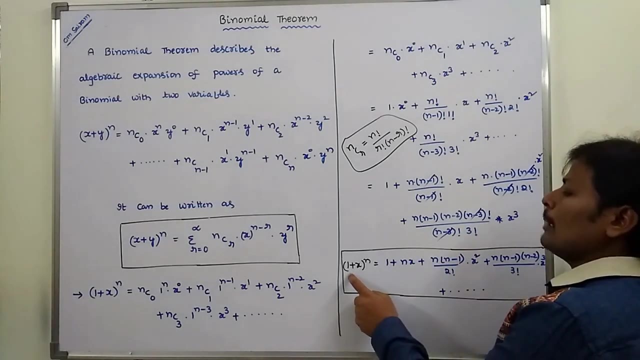 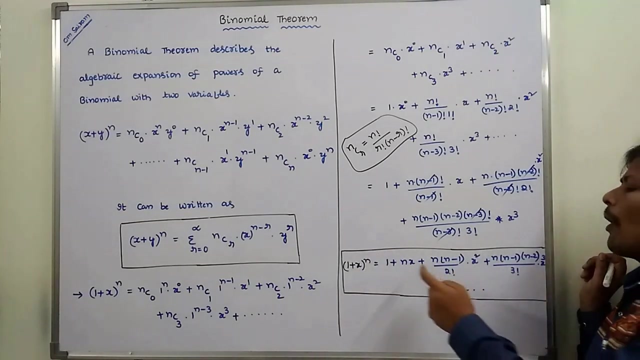 power n is equal to 1 plus n. x plus n into n minus 1 by 2 factorial into x. square plus n into n minus 1 into n minus 2 by 3 factorial into x cube. okay, this is the term. suppose 1 minus x whole power n, let the 1 plus x whole power minus n. is there so alternative terms? 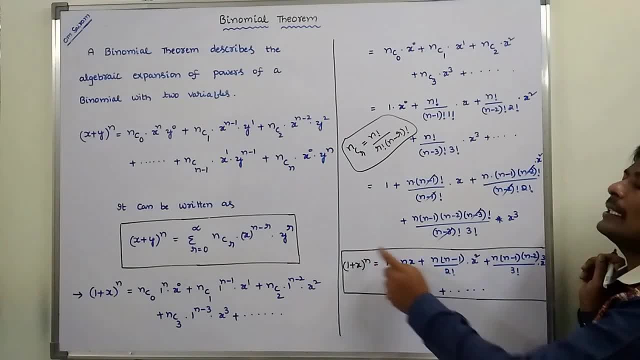 are minus, we are getting because the power contains minus value. so then alternative terms are negative. okay, so this is the description about the binomial theorem. so binomial theorem contains two variables, so either x plus y whole power n, or r, 1 plus x whole power n. okay, so on this binomial theorem we have to solve some. 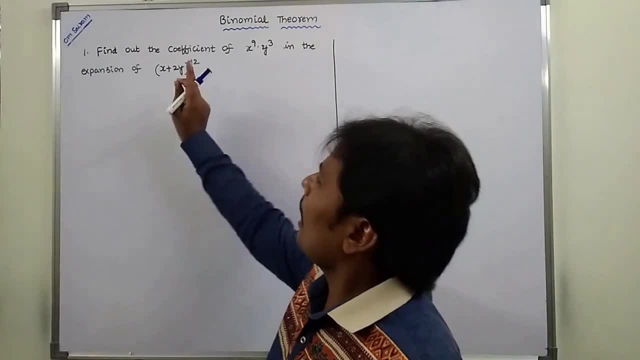 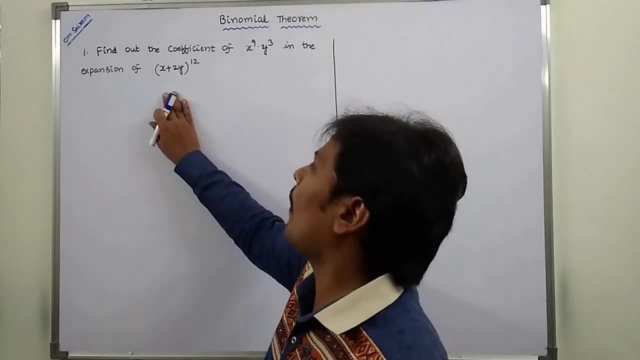 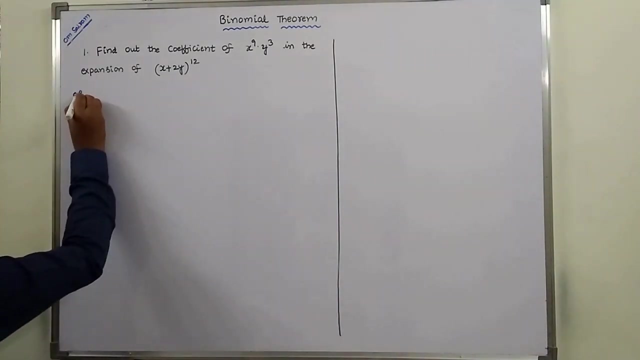 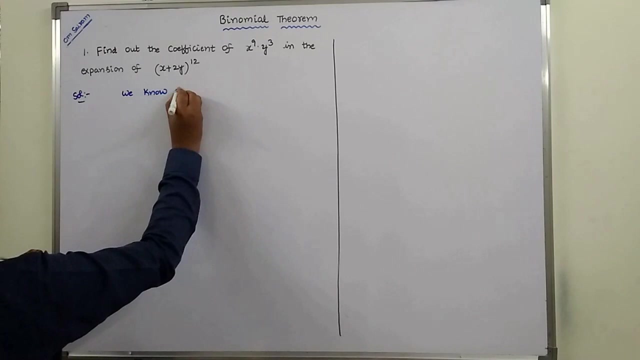 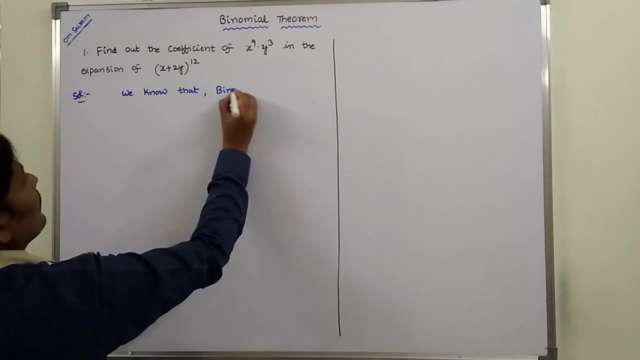 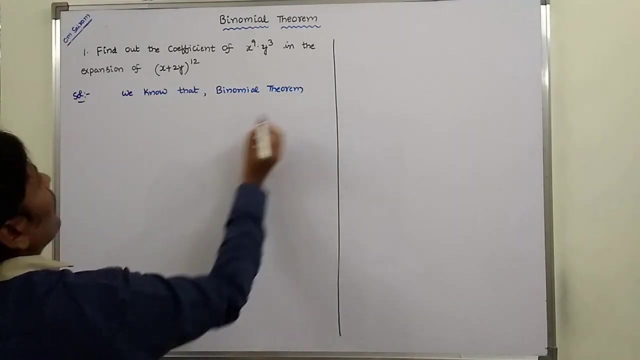 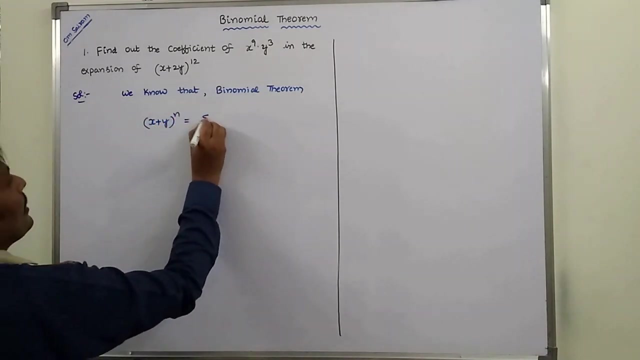 problems. okay, so find out the coefficient of x power 9 into y power 3 in the expansion of x plus 2y whole power 12. okay solution, we know that. we know that binomial theorem x plus y whole power n is equal to sigma, r is equal to 0 to infinity. 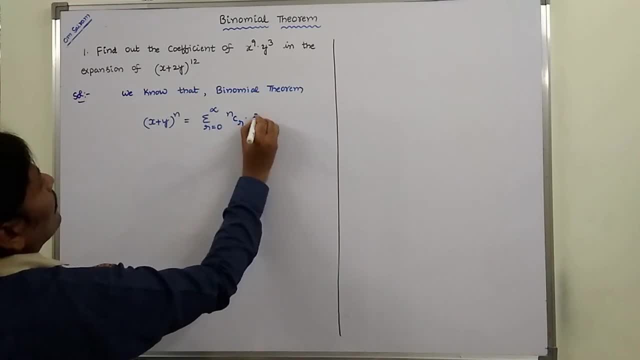 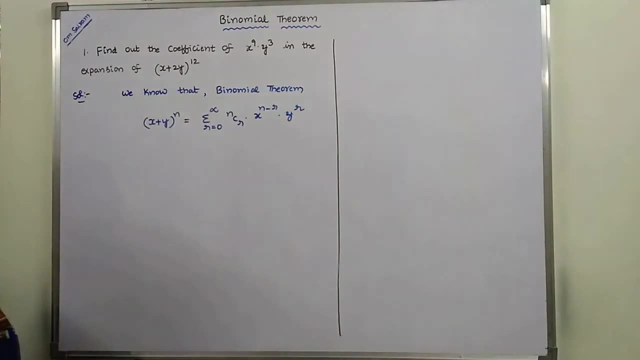 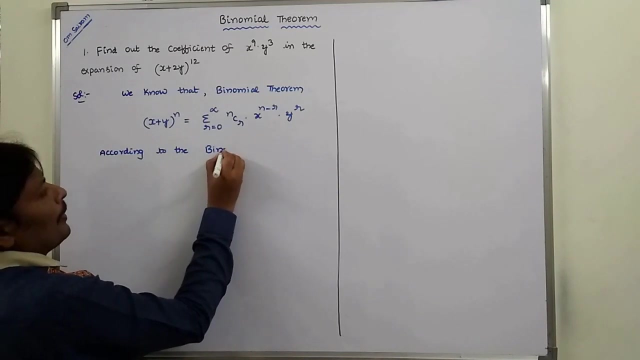 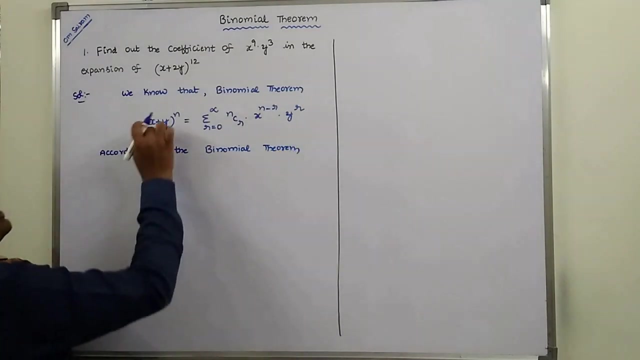 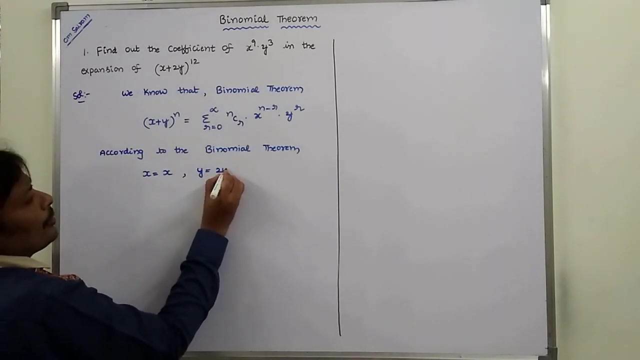 n plus y, whole power n is equal to sigma, r is equal to 0, to infinity. n nCr into x power n minus r into y power r. Okay, So, according to that, according to the binomial theorem, binomial theorem, so x is equal to x, y is equal to 2y, n is equal. 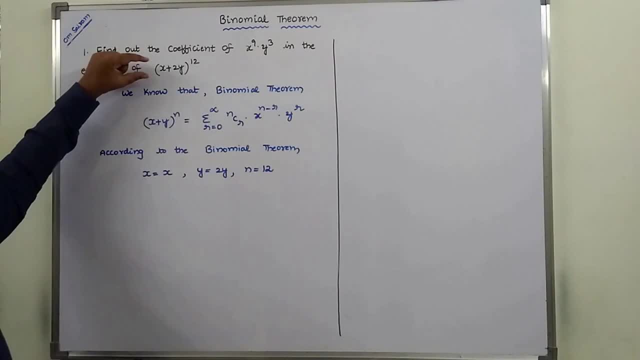 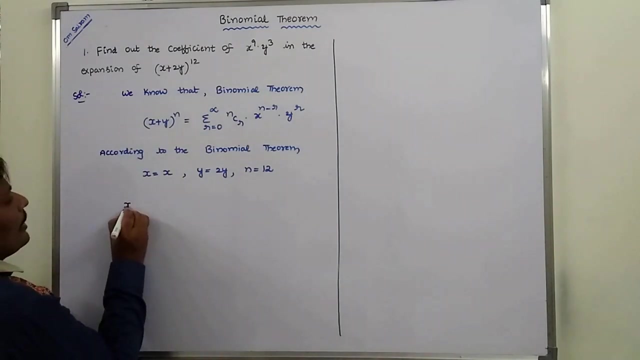 to 12.. Okay, Comparing this one is compared with this one, So we are getting: x is equal to x, y is equal to 2y, n is equal to 12.. Okay, So therefore, according to that, x plus 2y, whole power, 12, is equal to sigma. r is equal. 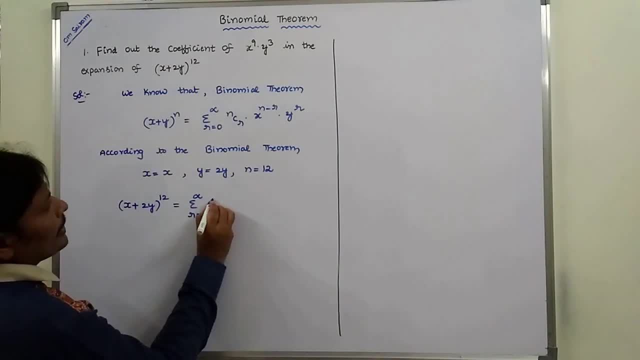 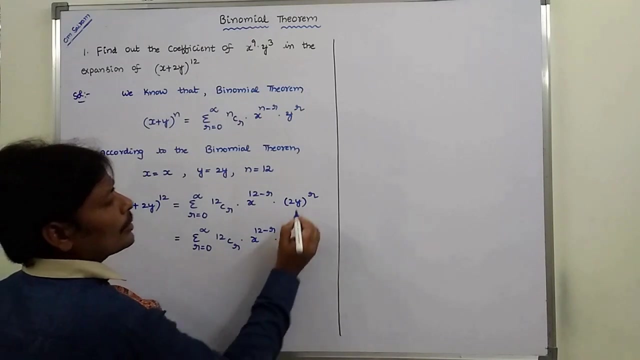 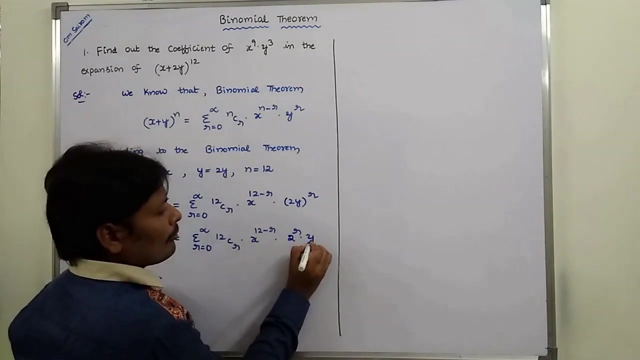 to 0 to infinity. nCr. 12Cr into x power n value: 12 minus r. Okay, So we can say: sigma r is equal to, sigma r is equal to. sigma r is equal to 0 to infinity. 12Cr into x power, 12 minus r into. so this can be written as: 2 power r into y power r. 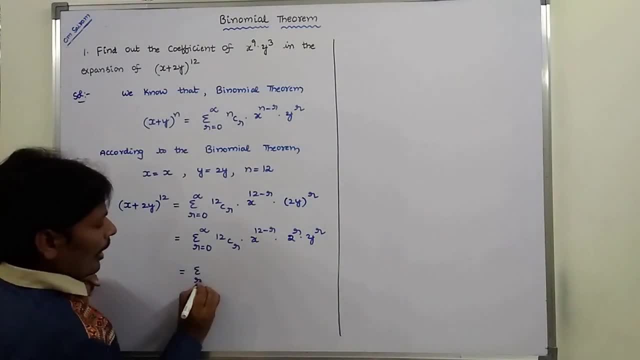 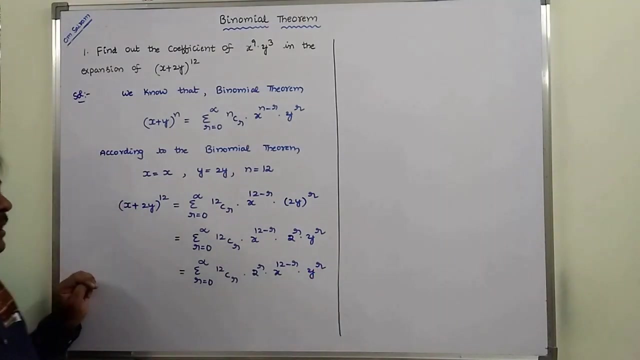 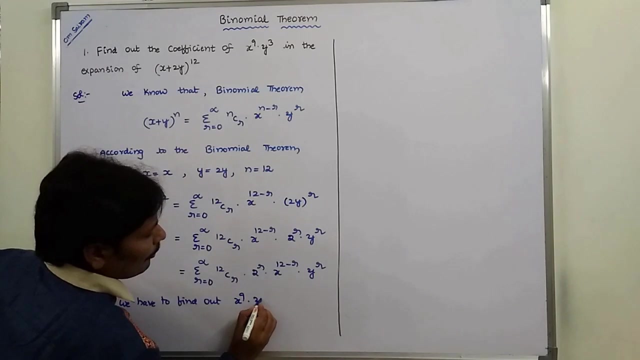 Okay, so then sigma r is equal to 0 to infinity. 12cr. x power 12cr into 2 power r into x power 12 minus r into y power r. Okay, so we have to find out x power 9 into y power 3.. 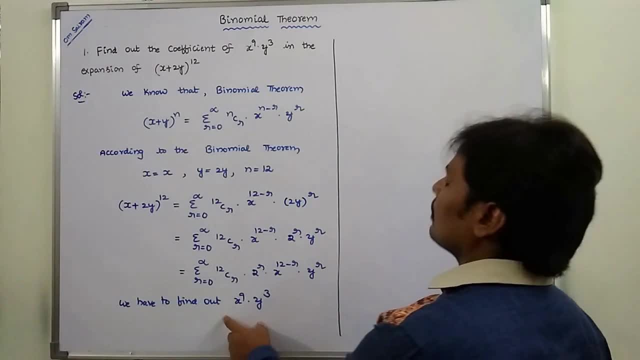 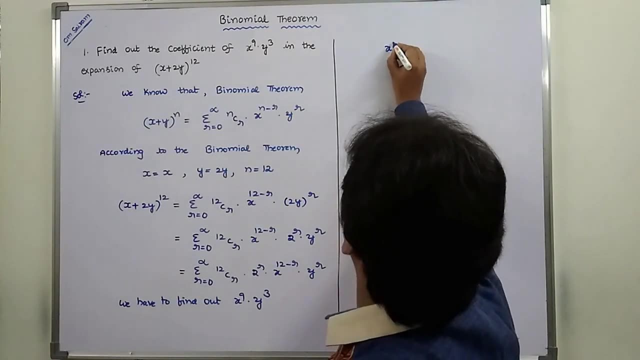 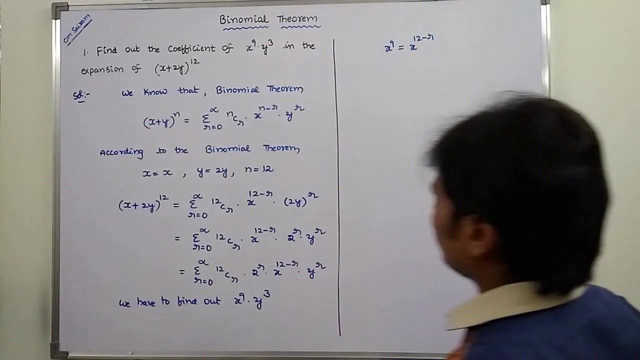 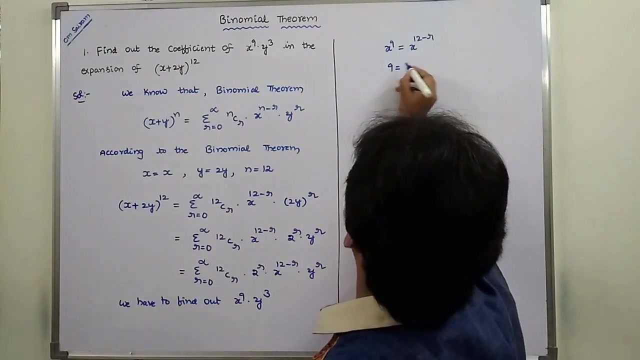 Okay, so now x term and y term are compared with this one. So we know that x power 9 is equal to x power 12 minus r comma. So bases are same. Then powers are equated: 9 is equal to 12 minus r. 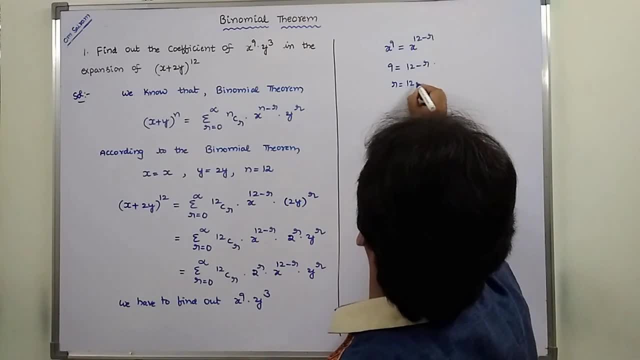 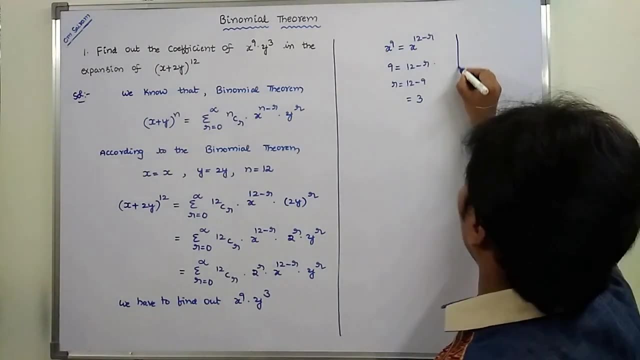 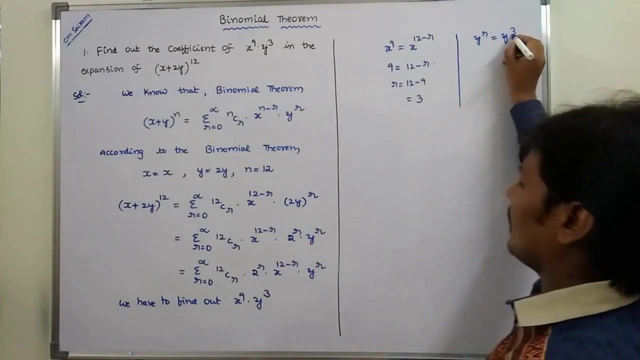 So therefore r is equal to 12 minus 9.. So that is equal to 3.. Okay, next one, Second one: y power r. So y power r is equal, is equal to y power 3. Here y power r is there. 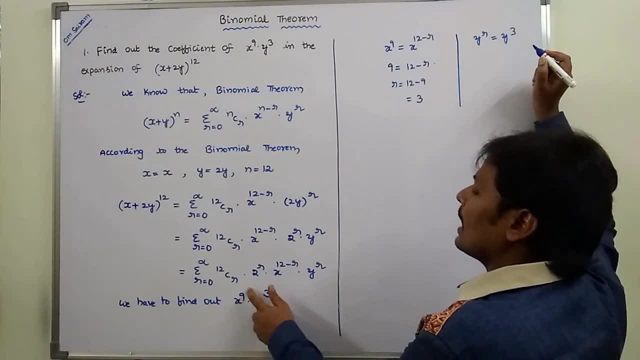 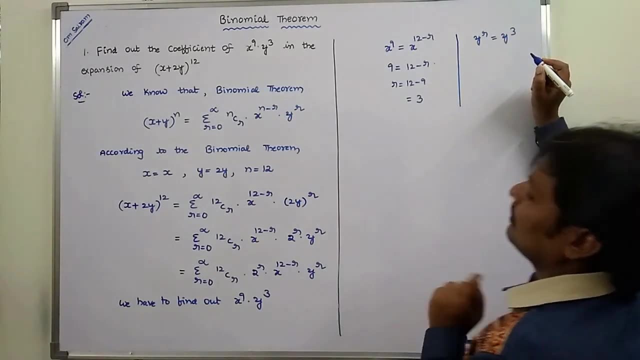 We have to find out y power 3. x power 9 into y power 3. So x term is equated with x term, Y term is equated with y term. So x term, x power 12 minus r is equal to x power 9.. 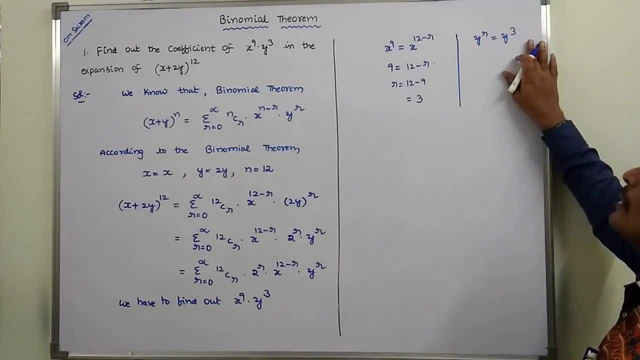 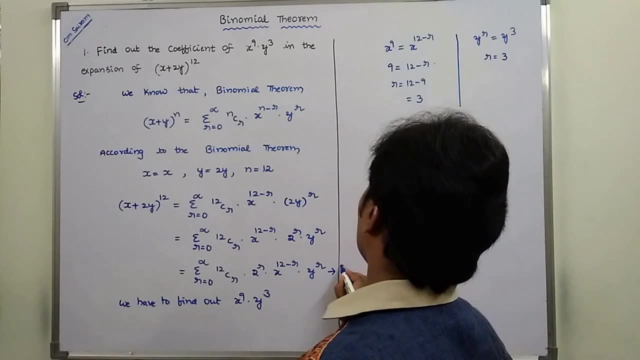 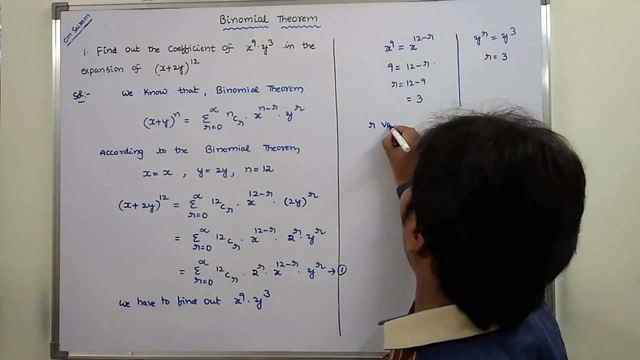 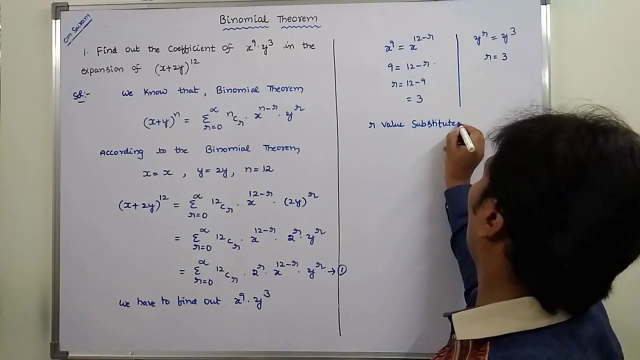 So y power 3 is equal to y power r. So according to that, so r value is equal to 3.. So now this is equation 1.. Okay, So r value substituted in equation 1.. In equation 1.. 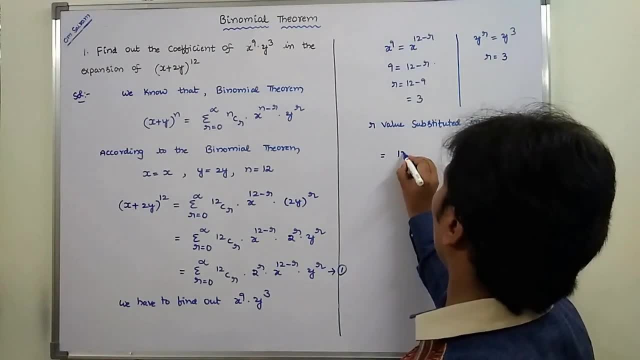 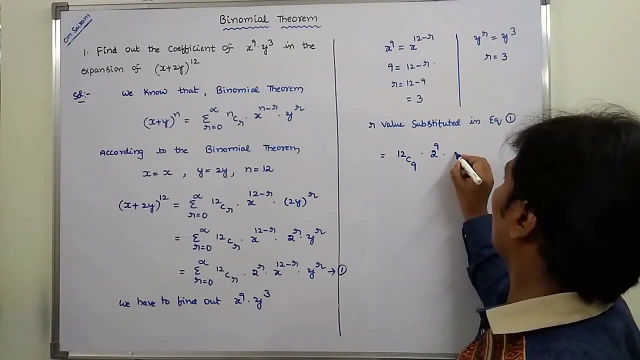 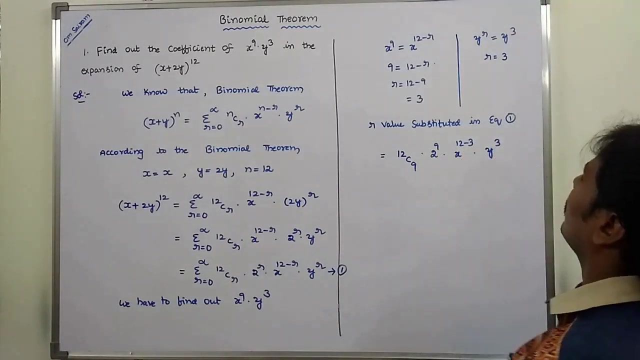 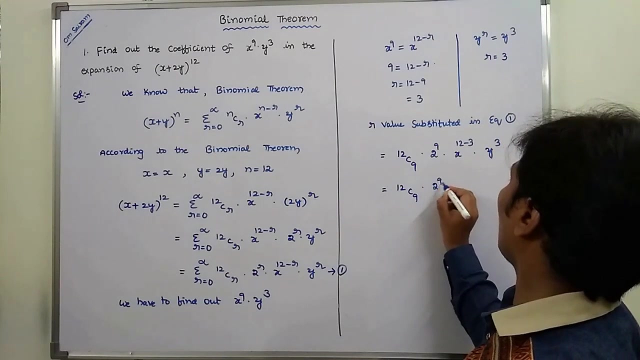 So therefore, 12c9 into 2 power, 9 into x, x power, 12 minus 3 into y power 3.. Okay, So then 12c9 into 2 power, 9 into x power, 9 into y power 3.. 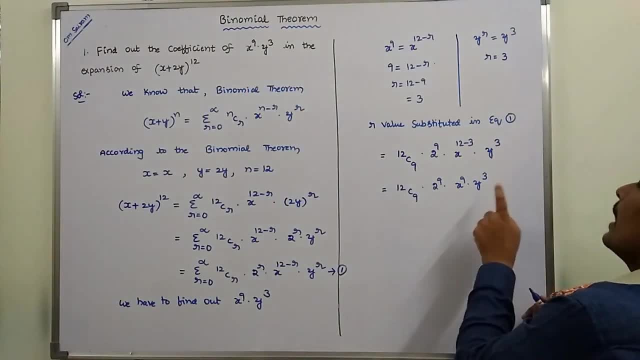 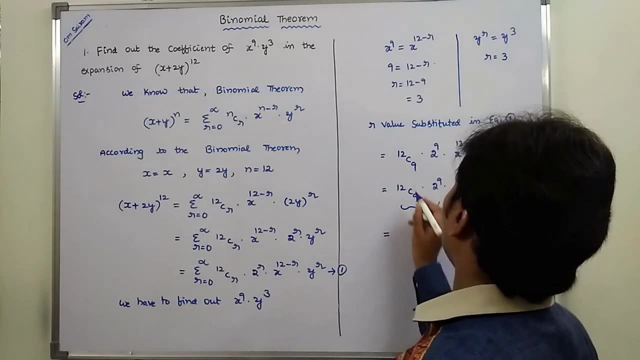 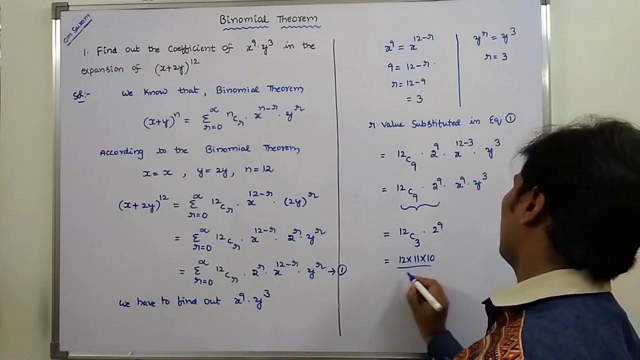 So we have to find out x power 9 into y power 3.. So the coefficient is this one. So therefore 12c9 can be written As 12c3 into 2 power 9.. So that is 12 into 11 into 10, divided by 1 into 2, into 3.. 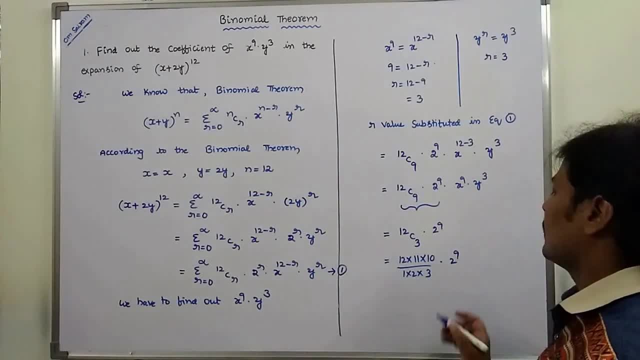 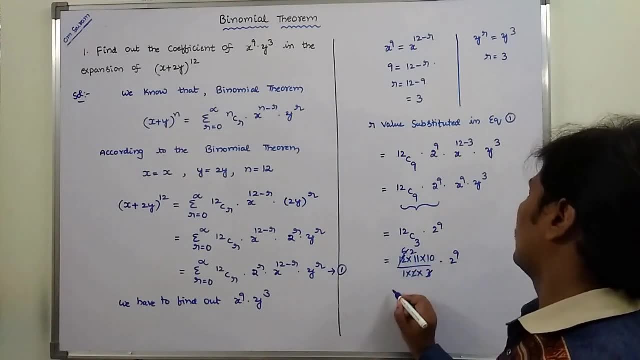 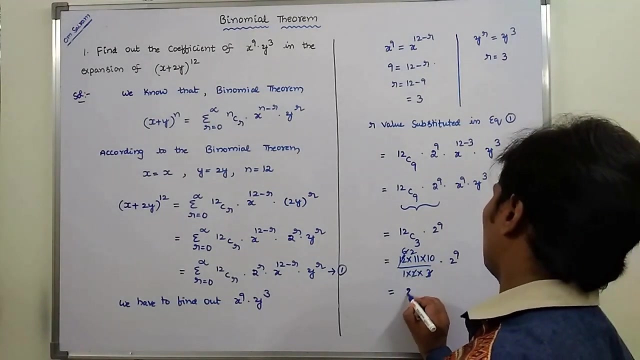 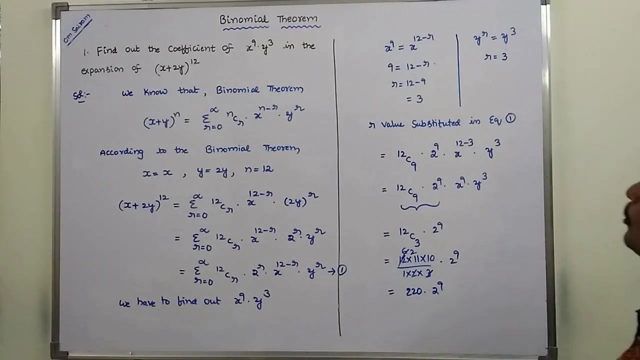 Okay, Into 2 power 9.. So 2, 6, 3, 2s. So 2 into 10, 20, 20. Into 11. 220. into 2 power 9.. Sorry, 2 power r. 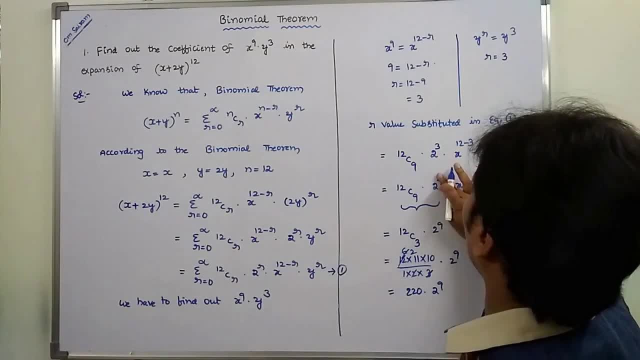 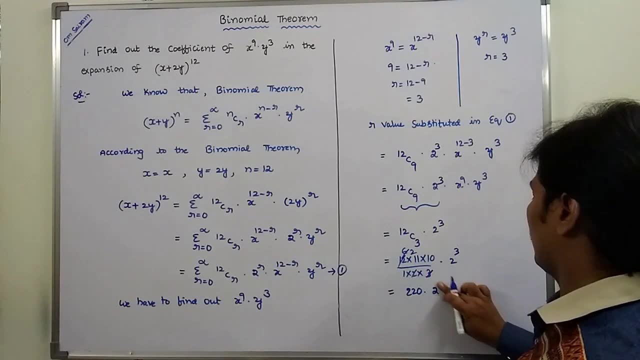 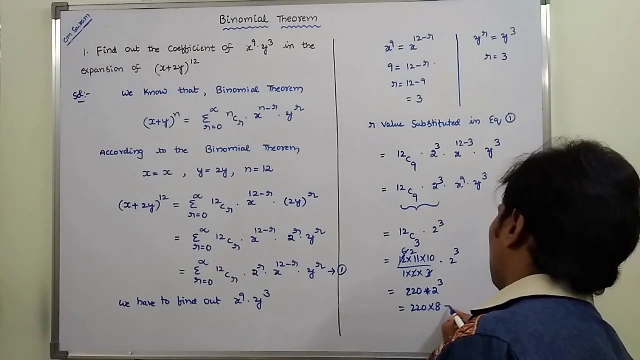 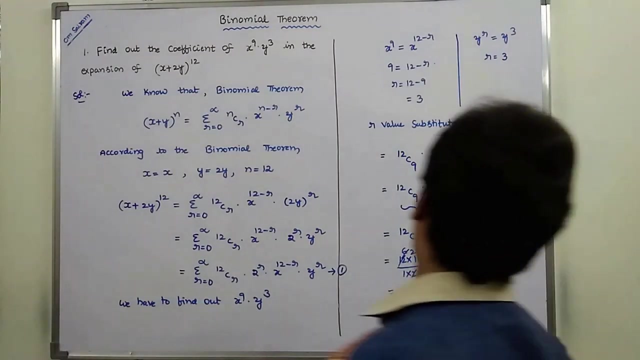 2 power r is 3.. So 2 power r is 3.. 2 power r is 3.. So 2 power r is 3.. So therefore, 220 into 8 is equal to 9.. eight zero, zero, eight, two, sixteen, that is seven, sixty. so therefore this is the. 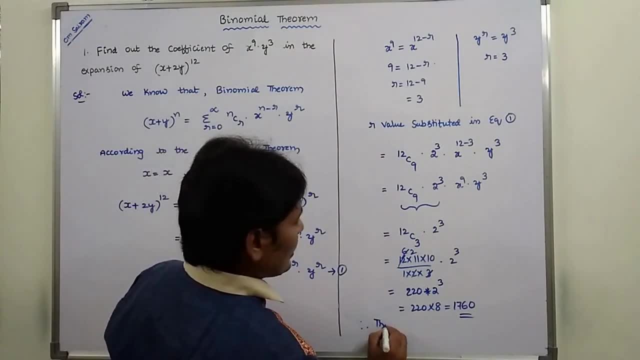 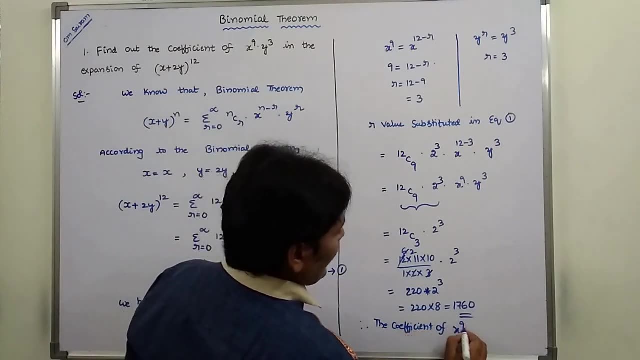 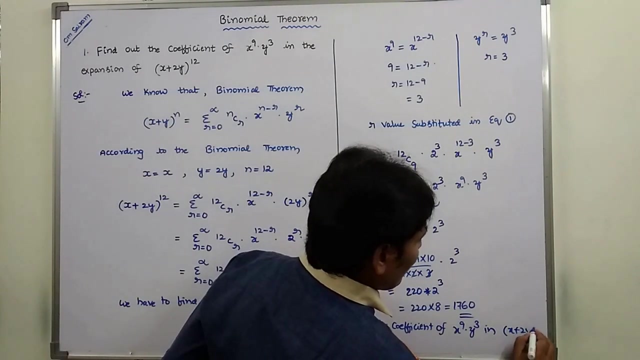 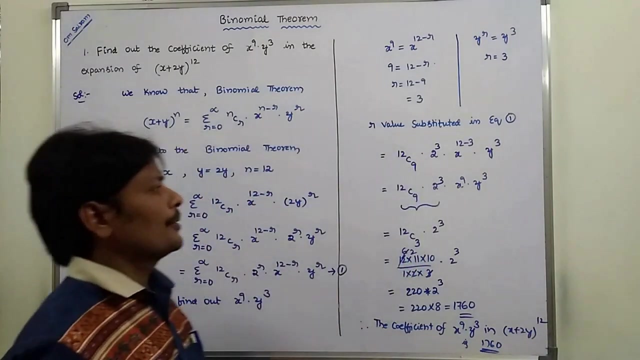 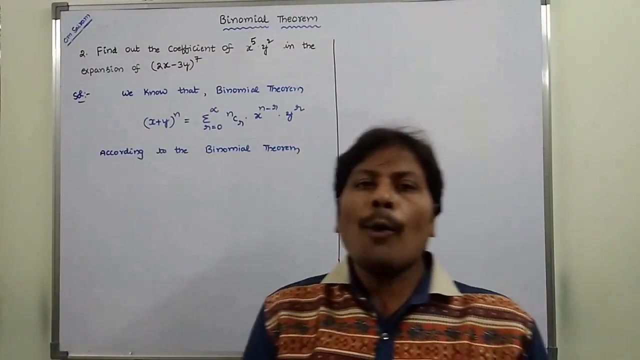 answer therefore: the coefficient of X power nine into Y power, three in X plus two Y, whole power 12 is 1760. so in this way we have to solve binomial theorem problem. now we go for second problem. find out the coefficient of X power 5. 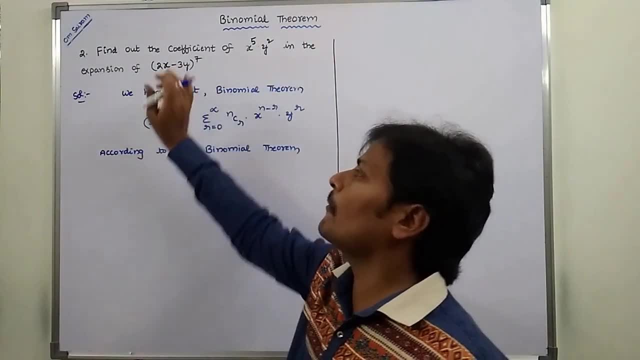 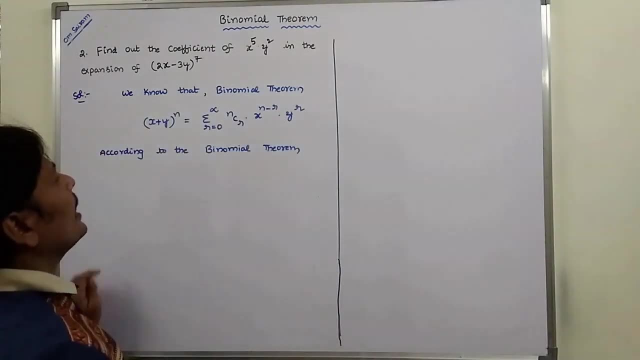 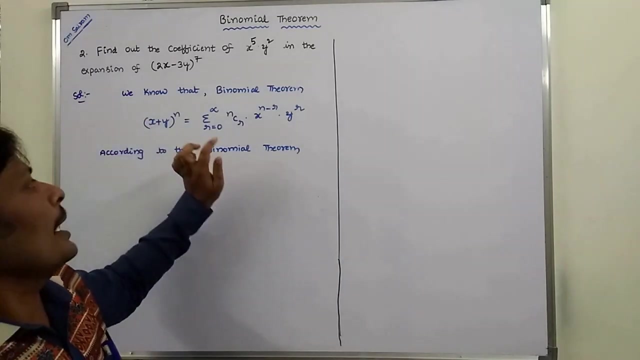 into Y power 2 in the expansion of 2x minus 3 by whole power 7. okay, so we know that the binomial theorem is X plus Y, whole power n is equal to sigma, r is equal to 0, to infinity MCR into X power n minus R, into Y power R. so 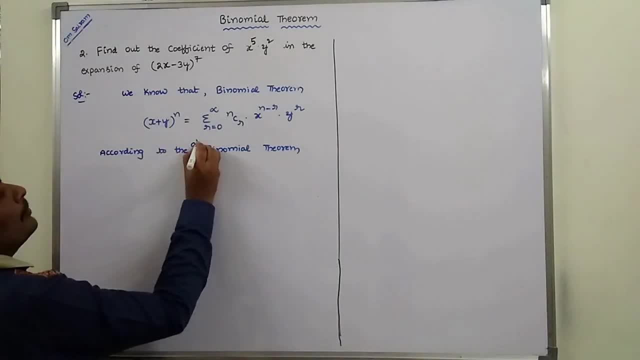 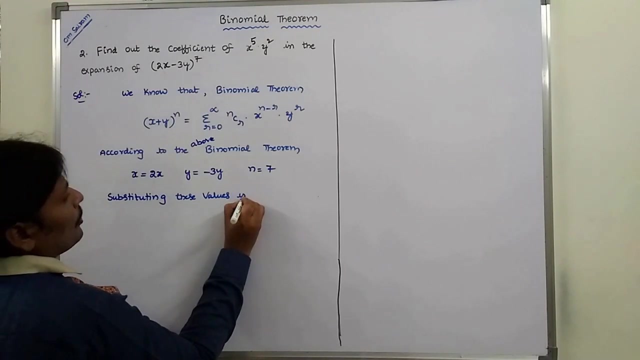 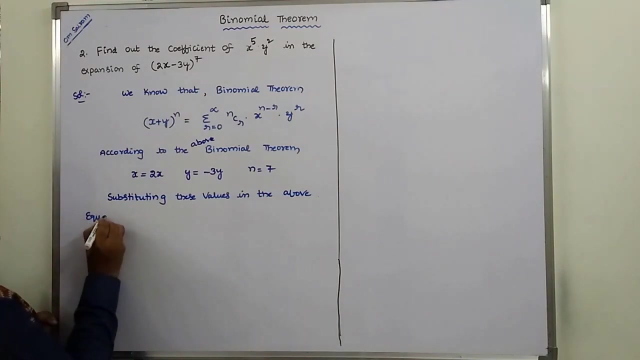 according to the above binomial theorem. so X value is equal to 2x and Y value is equal to minus 3y and the n is equal to seven. okay, so substituting these values, substituting these values in the above equation, in the above equation, okay, so 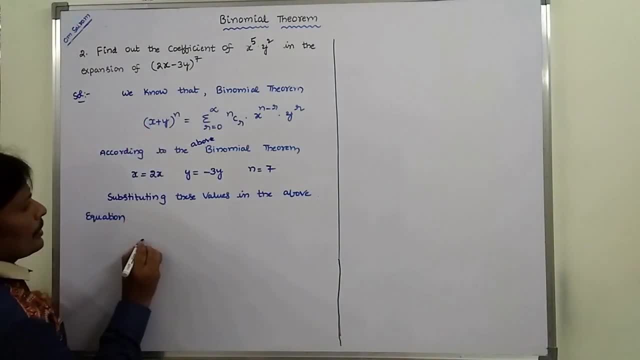 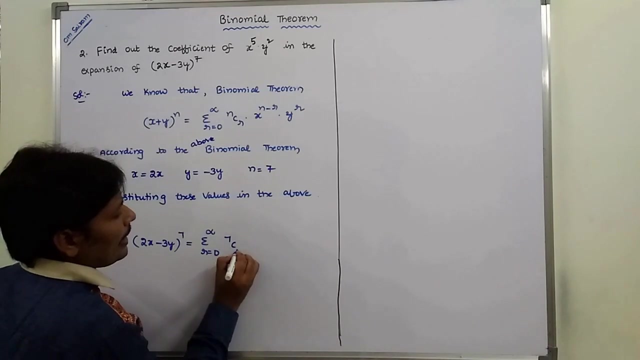 according to that X value 2x 2x minus 3 y, whole power 7 is equal to Sigma, R is equal to 0, to infinity. NCR, N value 7. so 7 CR into X power. X value how much 2x 2x? 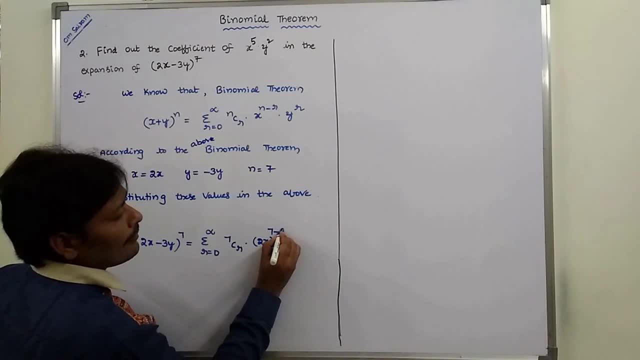 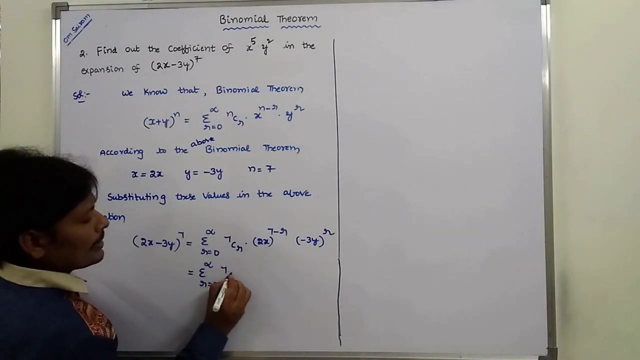 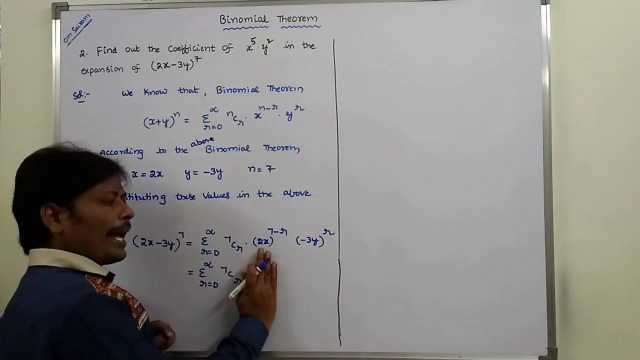 whole power: n minus on n value: 7, 7 minus R. Y power r. My value is minus 3y whole power r. Okay, So then sigma r is equal to 0 to infinity 7cr into. so this can be divided. this can be separated. this can be separated into two terms: 2 power: 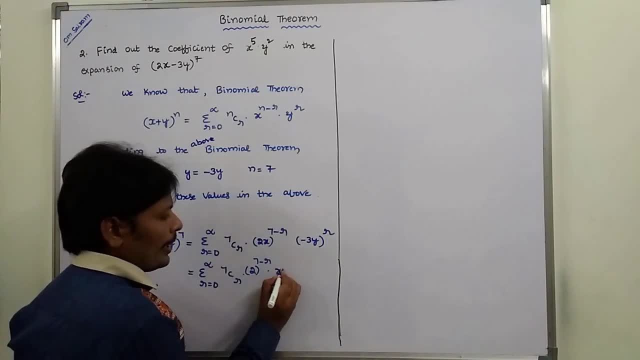 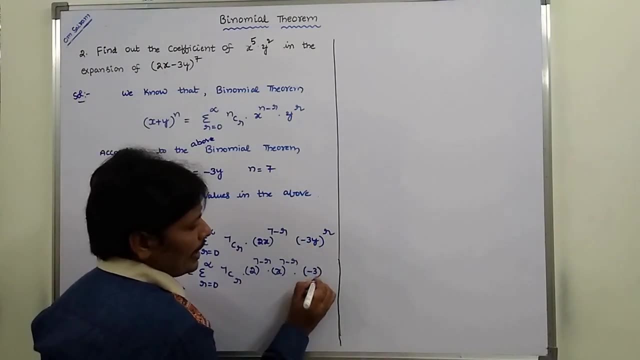 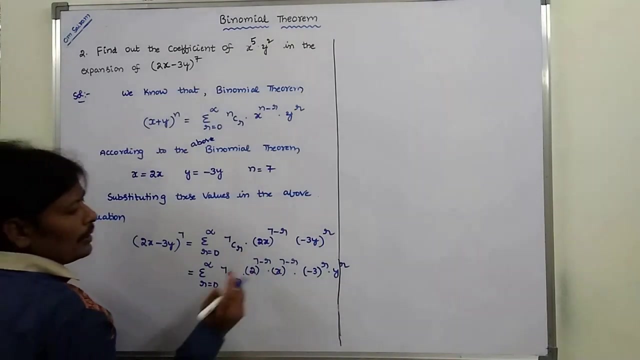 7 minus r into x power. 7 minus r. Okay, Again, this term can be separated minus 3 power r into y power r. Okay Now, constant terms can be separated one side, and x and y terms can be separated other side. Sigma r is equal to 0, to infinity. 7cr into x power. 7 minus r into x power. 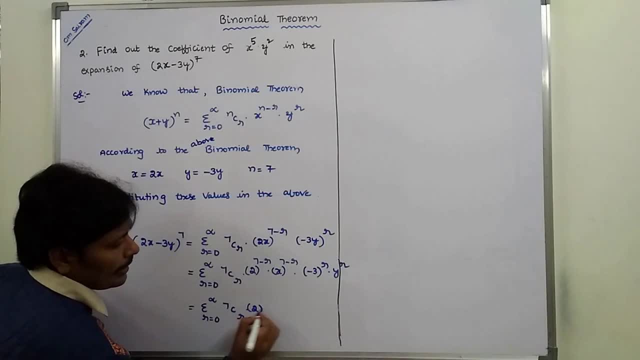 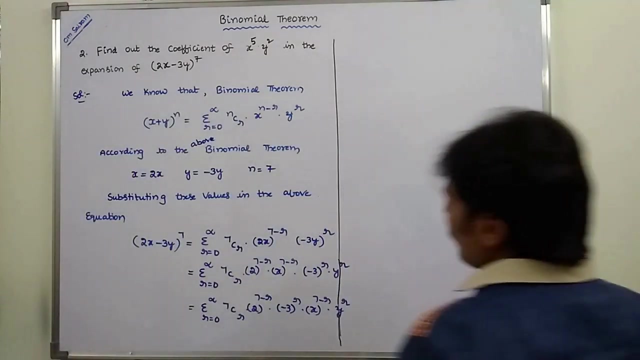 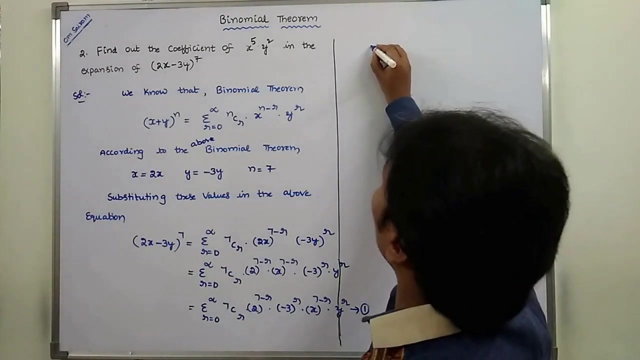 7cr into 2 power 7 minus r into minus 3 power r into x power 7 minus r into y power r. Okay, So now this is equation 1.. Okay, We have to find out the. we have to find out the. 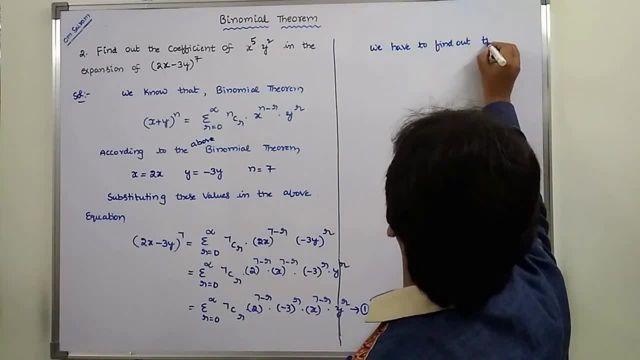 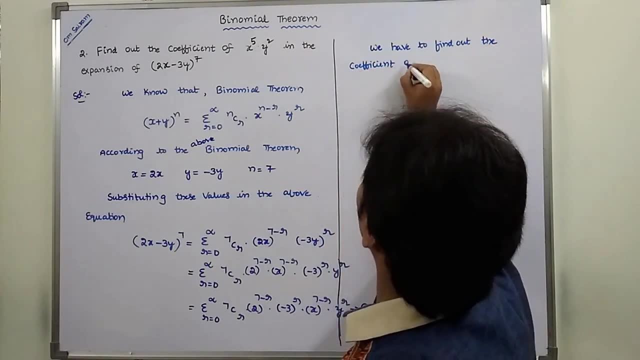 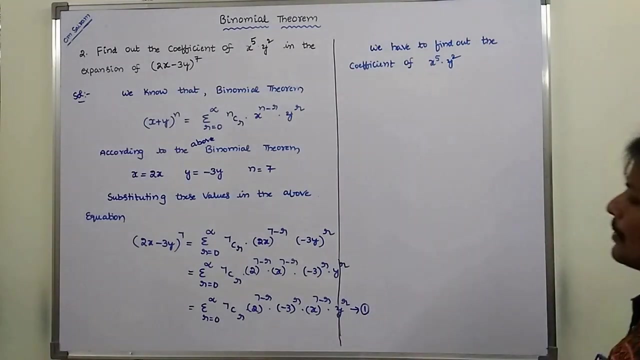 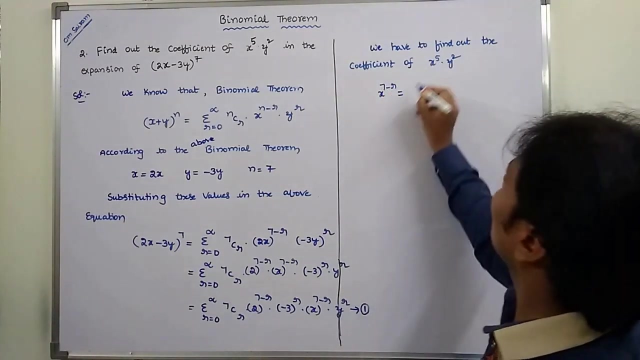 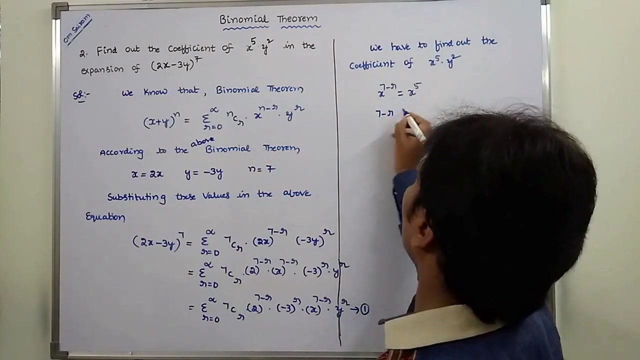 we have to find out the coefficient of, coefficient of x power 5 and y power 2.. Okay, So these x power term and y power term are compared with the equation 1.. So therefore, x power, 7 minus r is equal to x power 5.. So bases are equal, then powers are equal: 7 minus r is equal to 5.. 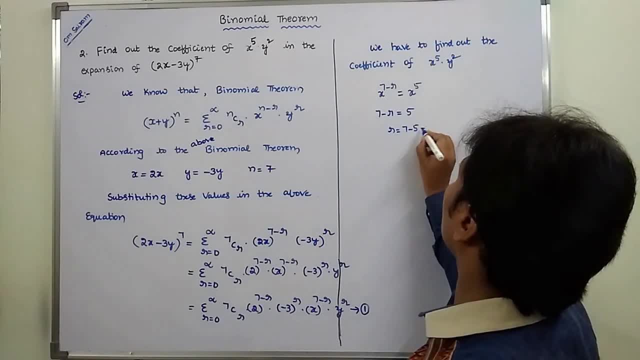 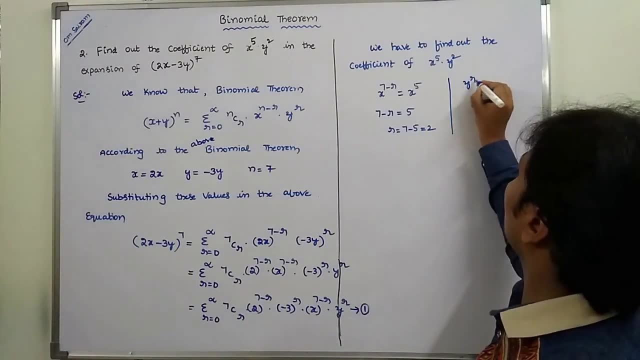 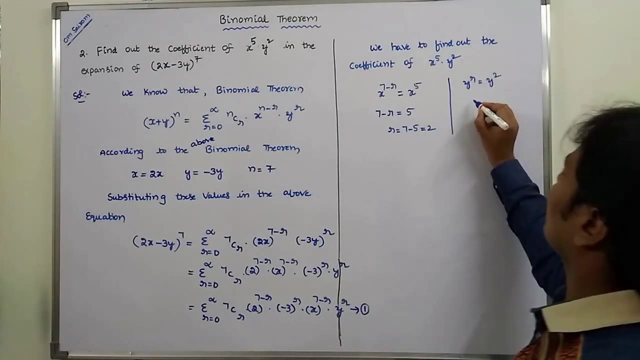 So r is equal to 7 minus 5, that is equal to 2.. Okay, In the same way, y power, r is equal to y power 2.. Okay, Y powers are equated with y power 2.. So therefore, r is equal to x power 2.. 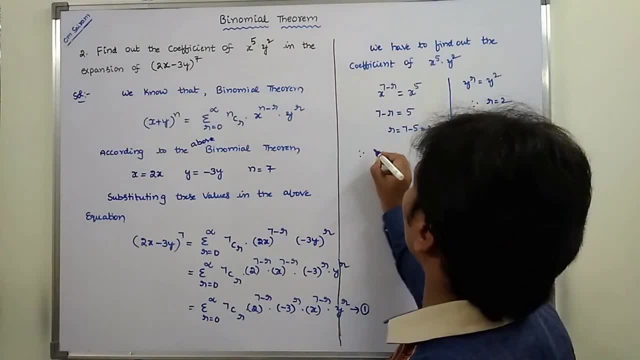 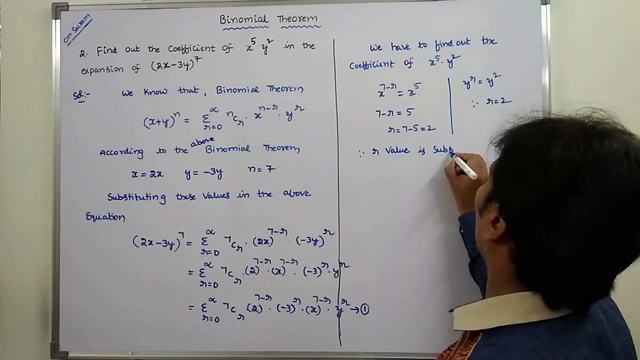 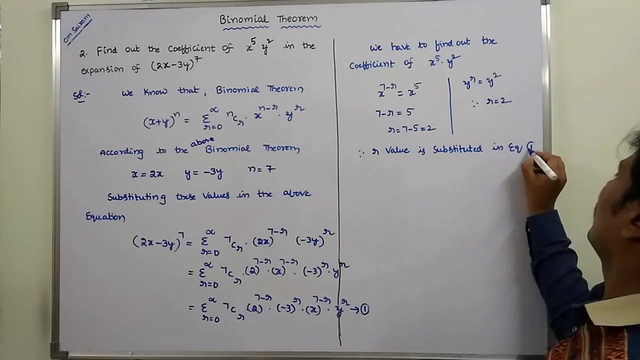 So then, what is the result? This is the part where you are going to are going to- is equal to twice ax power 3 plus x power 4 plus f power 6- sorry, k power 9 times 2.. So, at that moment, y power is equal to p power 1 wh-By circle. look at the everything. 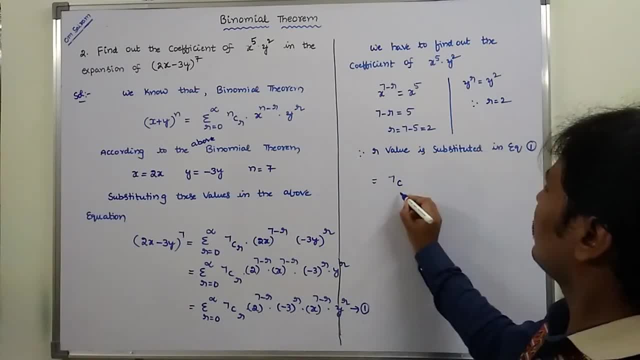 So y power times 2 times x power 3 equal to 1.. Okay, So research. everyone does not want to learn math And re今天的. survival is so important. That is why in cars, in cars, in cars is true. Now let's say the speed is equal to 1.. Opposite is equal to 1.. Same thing in car, in cars. in cars It is equal to 1.. So it is equal to 1 times x and x power 3, almost n. This the result is. by adding everything, the value comes out will be' It increase the power x power 2, because we are going to have 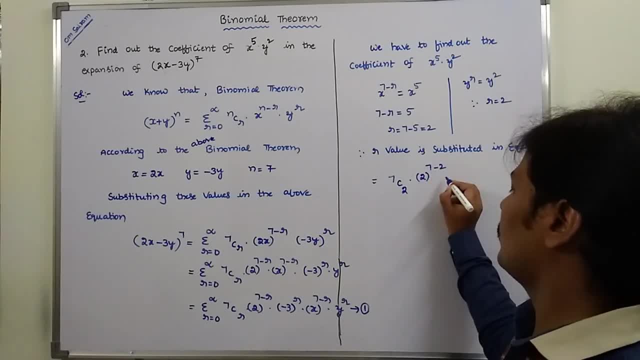 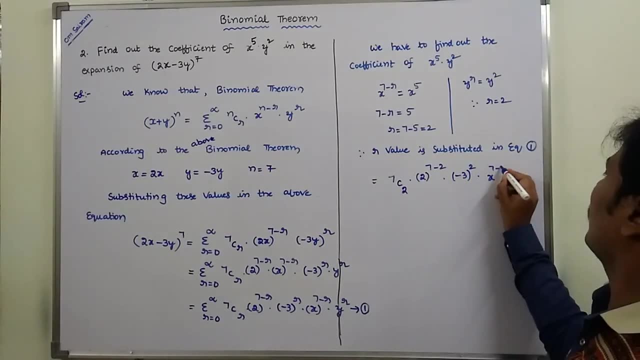 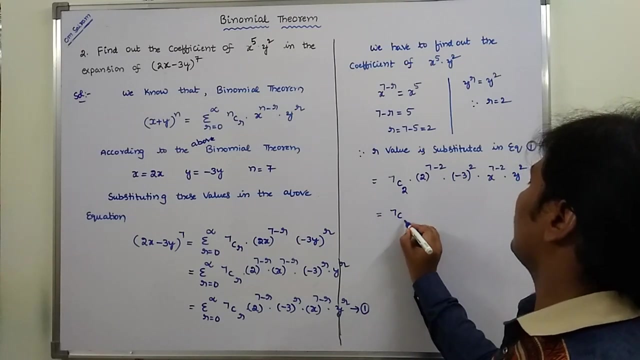 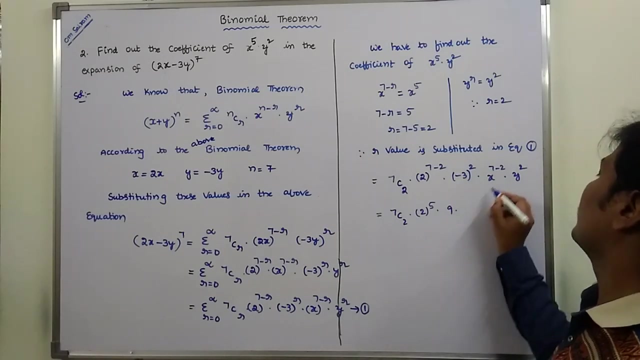 2. power 7 minus 2 into minus 3. power 2 into x. power 7 minus 2 into y power 2. okay, so that is equal to 7. c 2 into 2. power 5 into minus 3. power 2 is nothing but 9. so this is x power 5 into y. 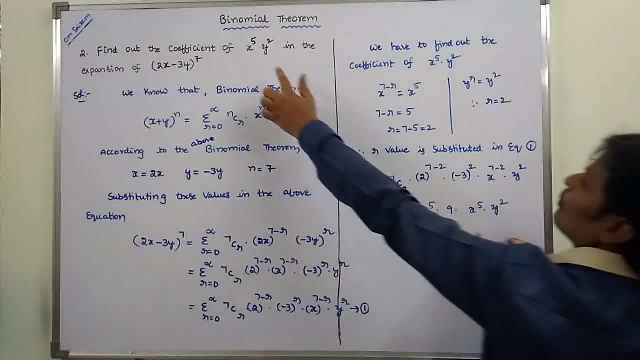 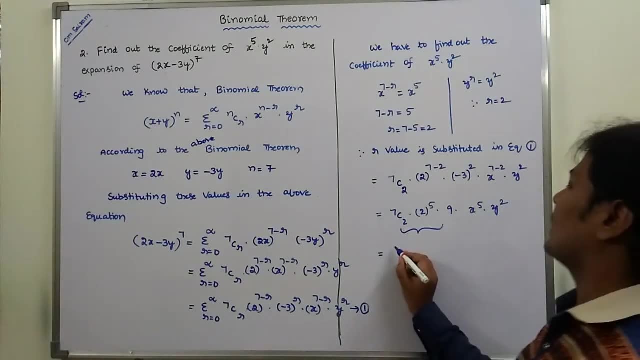 power 2. so we are getting x power 5 into y power 2. so this is the coefficient term. okay. so then, 7 c 2, 7 into 6, divided by 1 into 2 into 2, power 5 is 32, 32 into 9, into x power 5 into y power 2.